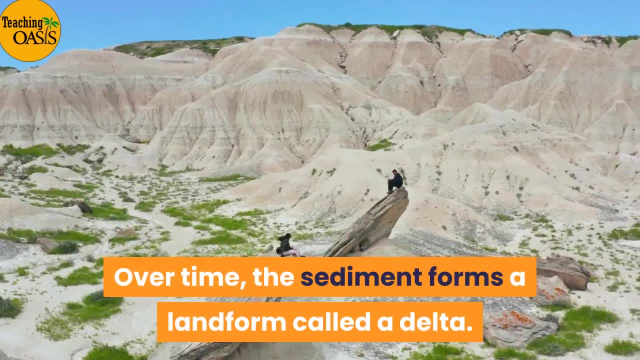 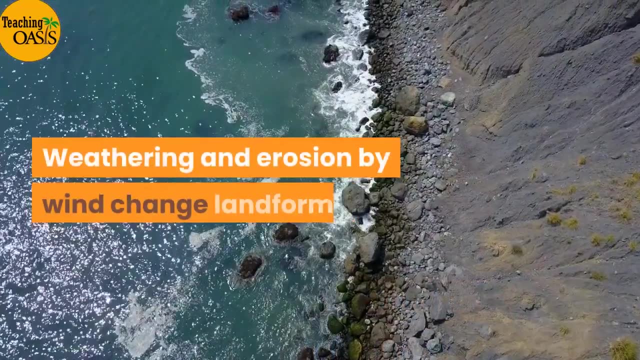 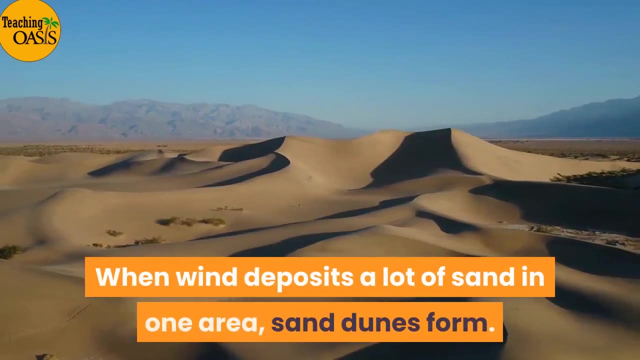 Over time the sediment forms a landform called a delta. Blowing in the wind, Landform is a natural land shape or feature. Weathering and erosion by wind change landforms. Wind can carry sediment from place to place. When wind deposits a lot of sand in one area, 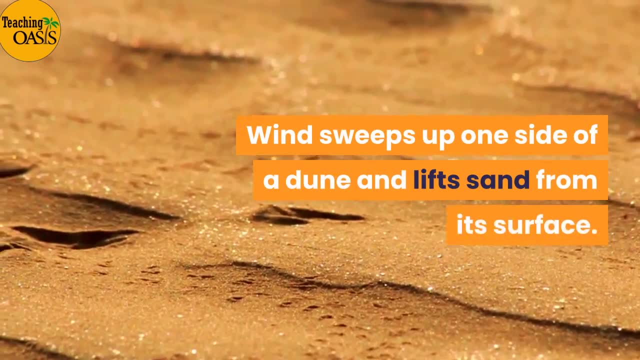 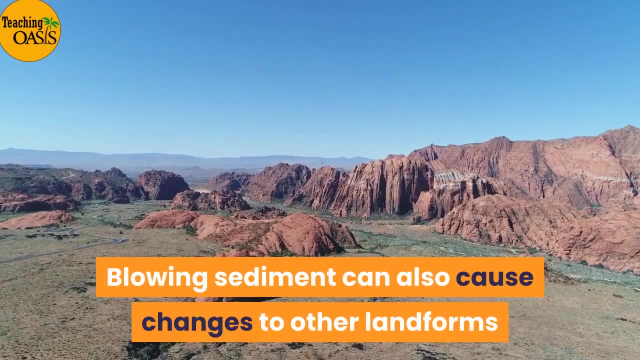 sand dunes form. Wind sweeps up one side of a dune and lifts sand from its surface. Gravity pulls the sand down the other slope. Blowing sediment can also cause changes to other landforms as particles collide with exposed rock to form interesting shapes. 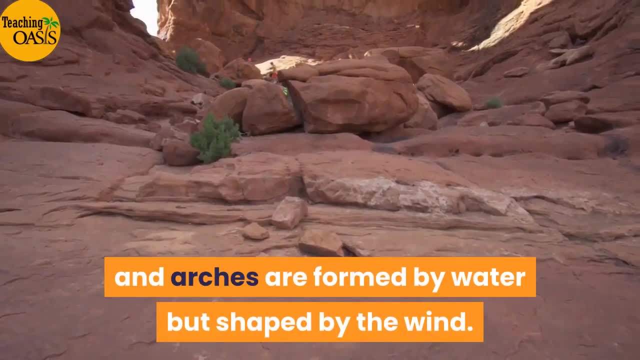 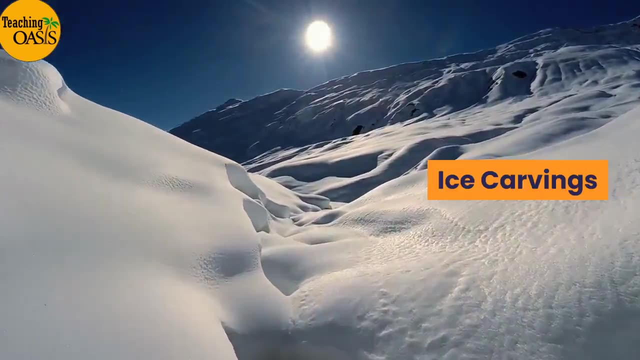 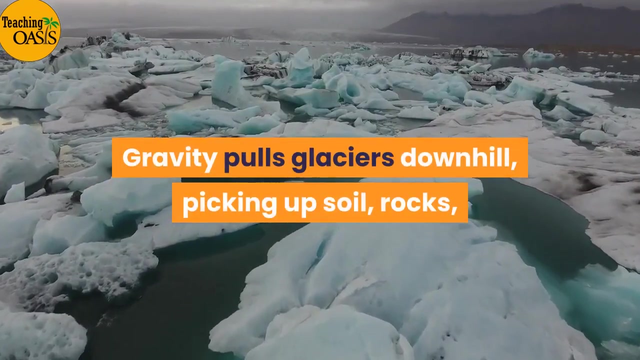 For instance, mushroom rocks and arches, are formed by water but shaped by the wind. Eventually, gravity pulls these formations down. Ice carvings, Huge sheets of ice, are called glaciers and are found in very cold places. Gravity pulls glaciers downhill, picking up soil, rocks and boulders beneath the glacier, and 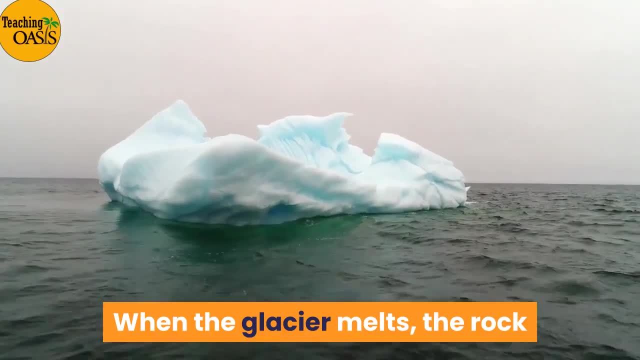 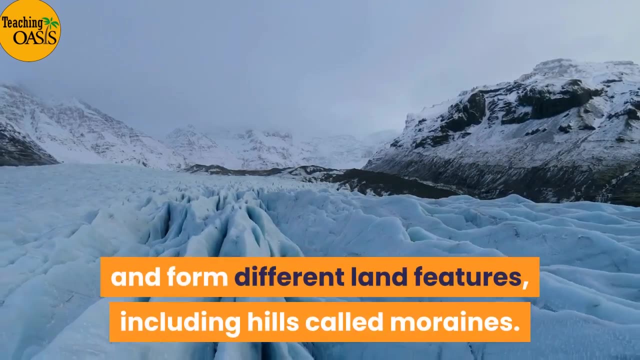 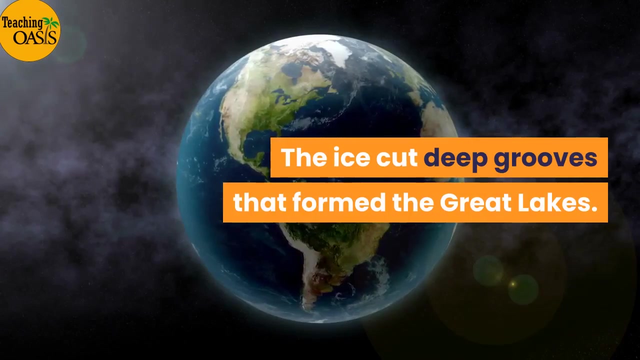 pushing boulders against the ground below. When the glacier melts, the rock and sediment it carried downhill drop out and form different land features, Including hills called moraines, A huge glacier once covered most of Canada and the northern United States, The ice cut deep grooves that formed the Great Lakes. 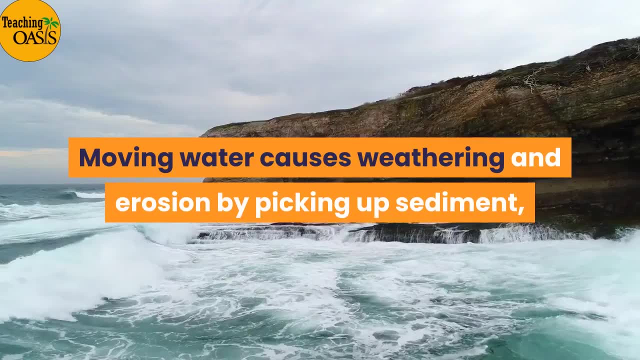 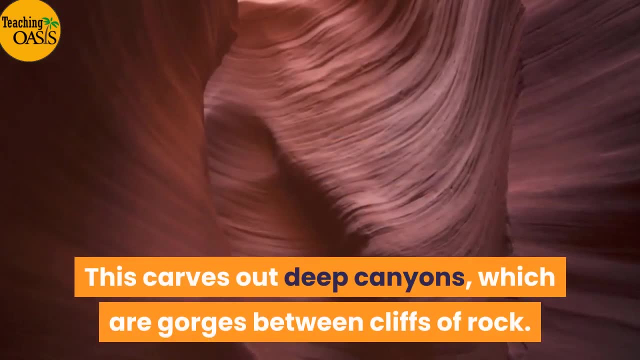 Can waves cut caves. Moving water causes weathering and erosion by picking up sediment which scrapes against the bottom and sides of the riverbed. This carves out deep canyons which are gorges between cliffs of rock. Deposits of sediment can change the direction of river water. 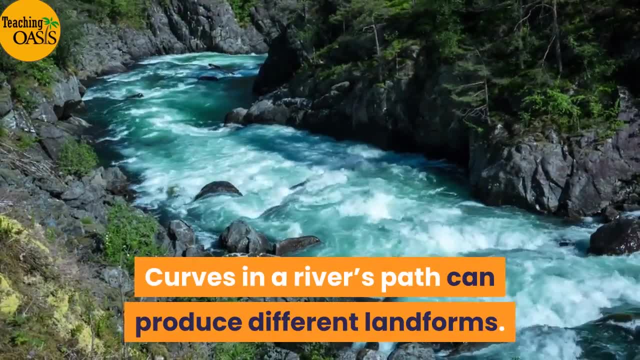 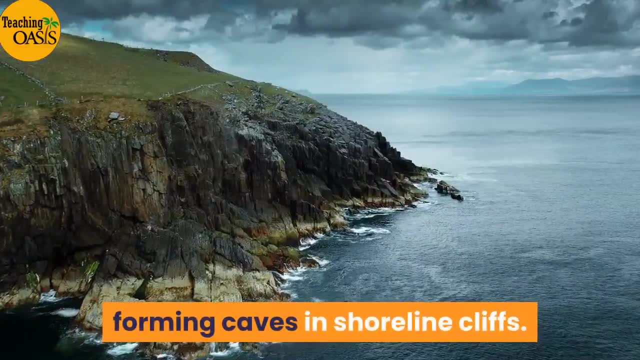 Curves in a river's path Can produce different landforms: Ocean waves, weather, cliffs, eroding pieces of rock and depositing them into new places, forming caves in shoreline cliffs. The sediment from eroding shorelines becomes fine sand and beaches are formed at the water's edge. 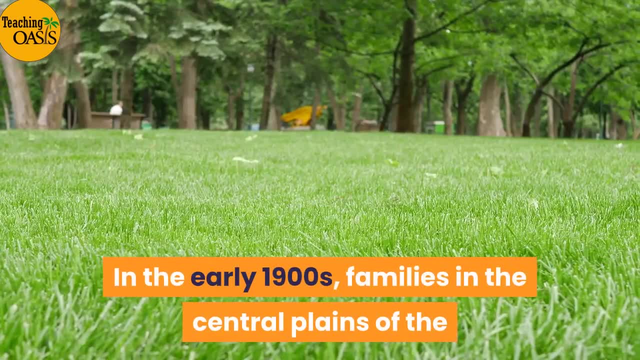 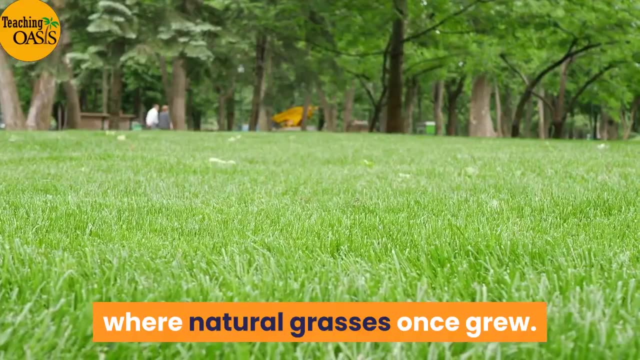 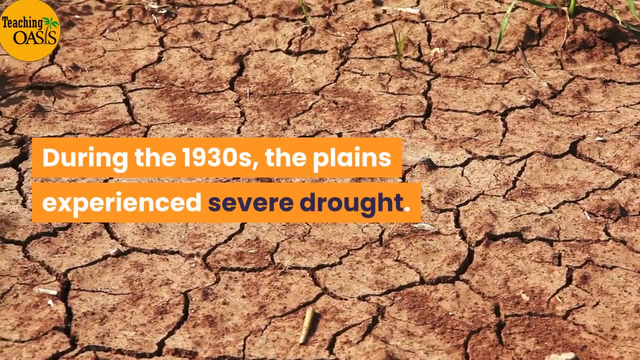 Do plants protect soil? In the early 1900s, families in the central plains of the United States made a living farming land where natural grasses once grew In. between crop seasons, loose soil soil was left exposed to wind. During the 1930s, the plains experienced severe drought.